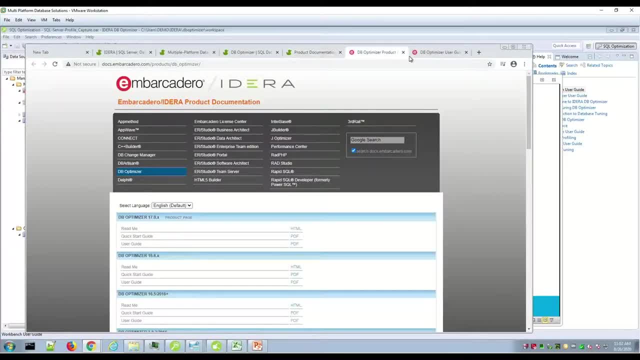 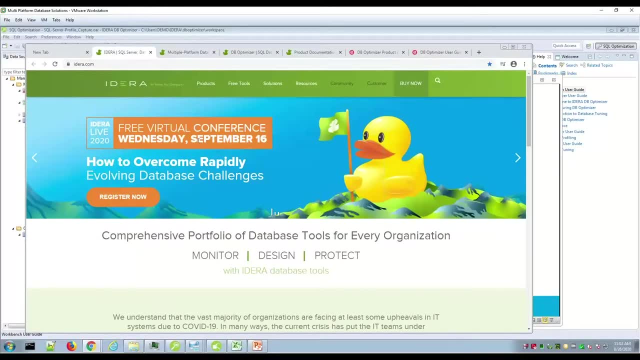 all the products in the PowerStudio bundle and and that those are helpful resources for you as well. So we'll show you some of these areas before we wrap up today, and then we'll get into some of those I also wanted to mention. we have the IDERA live conference next month or in three weeks on. 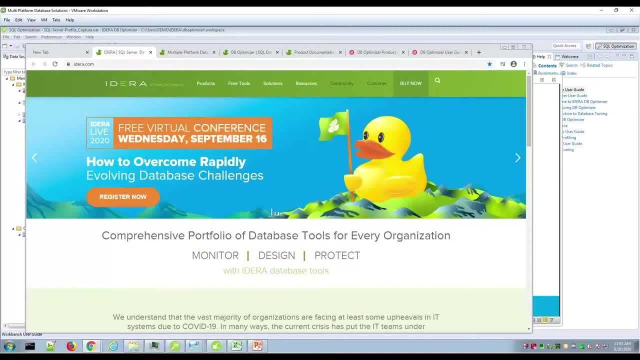 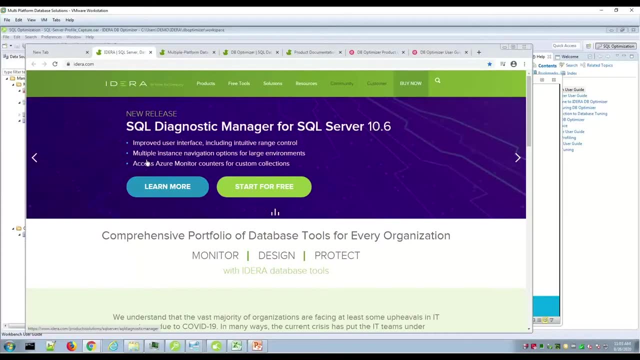 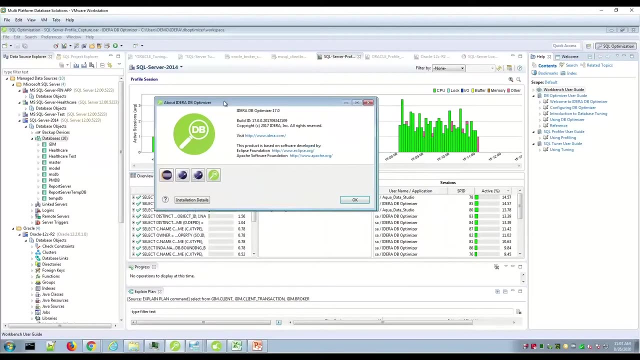 September 16th, so that's a day of seminars and product demonstrations, and so different, different ways to to dive in and take advantage of some of the solutions that IDERA offers for you. Okay, so I have the product open and so we'll introduce the user interface. this is a very mature technology. 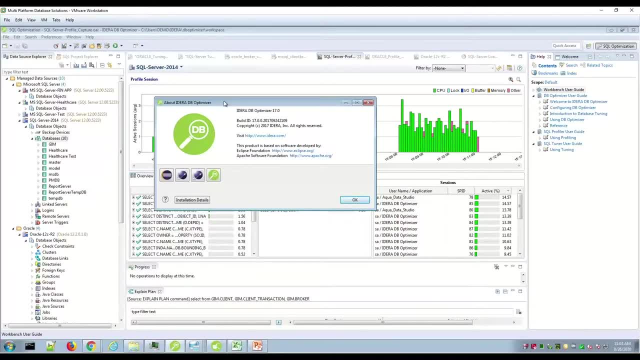 up to a version 17.. I've been on the market for over- you know, over a decade now, and I've been on the market for over 20 years and now has stayed current with the four major RDBMS platforms of SQL Server, Oracle, DB2, and Sybase. So you have resources here in terms of 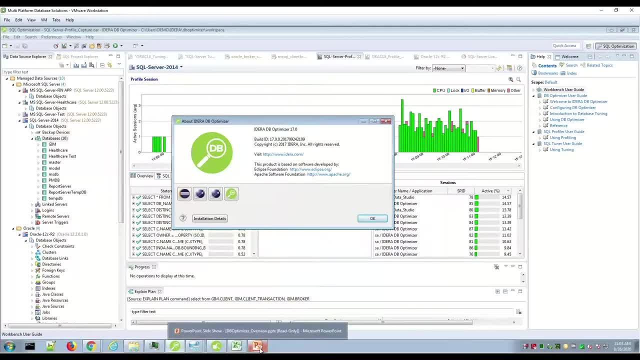 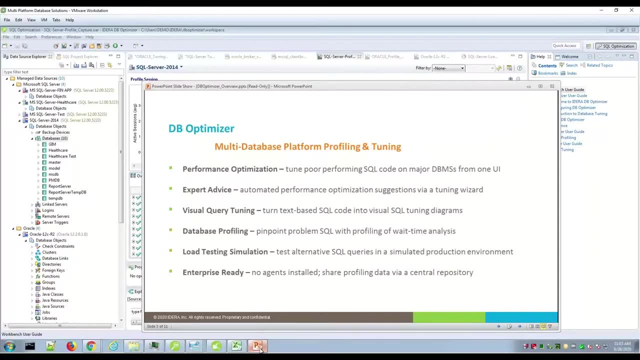 documentation and and more details on these areas, but here's just a few slides to introduce. where dbOptimizer can help- and we've built some of this from the documentation and and the tools named named- well, It optimizes the database and that can be in terms of performance and finding bottlenecks and doing. 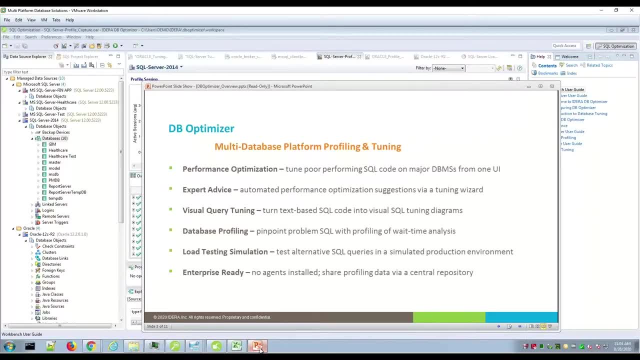 weight analysis or drilling down into individual SQL. and so if you, if you have SQL that you're interested in tuning, that that could be a starting point, right, so you can. you can dive right into SQL tuning If you are more interested in looking at performance or finding where the SQL that needs. 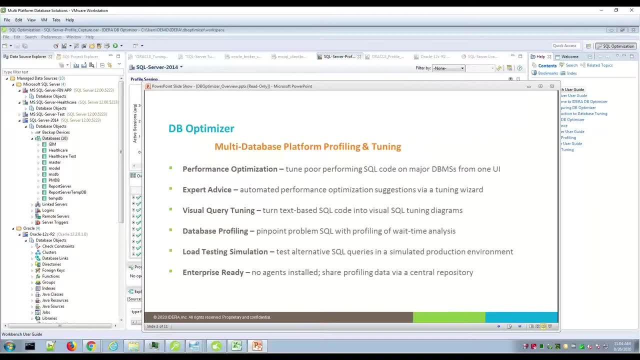 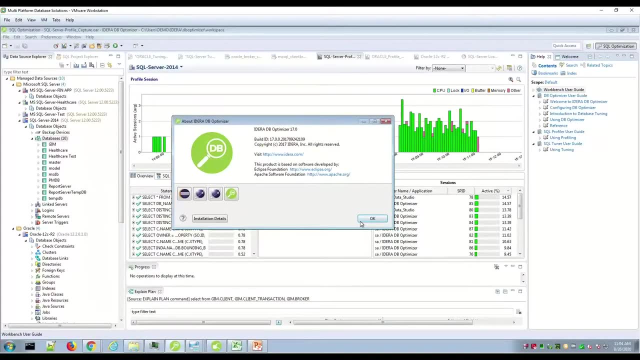 tuning is. that's the database profiling area. So those are the two areas that we'll focus on today, And then the documentation really focuses on that as well. So just here on the left hand side, or the right hand side rather, you can see i have SQL profiling, SQL tuning. so those are the two main areas that we'll look. 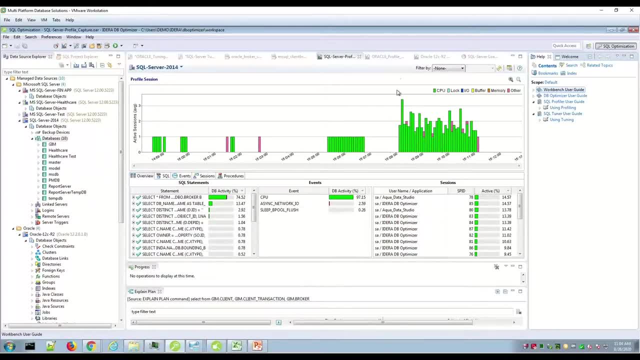 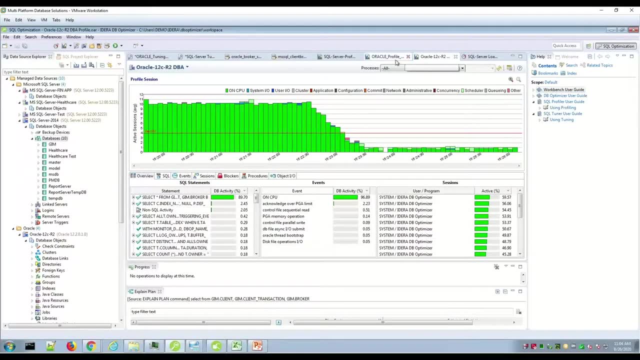 at here today. Here's an example of the, the profiling display. So here's a profiling collection in SQL Server, Here's a profiling collection in Oracle, or multiple in Oracle, and so that could be a starting point, right? This is where you you can do a capture and 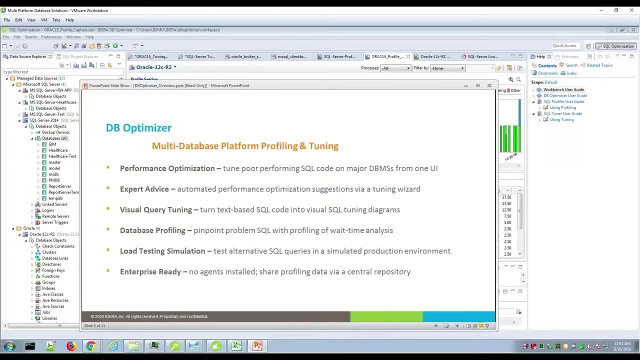 and collect SQL performance and transactions from your applications and then dive into optimizing SQL. If you know the SQL that you'd like to tune, you can dive right into the visual query tuning. And then there's different rewrite capabilities and then comparisons of the executions of those rewrites. 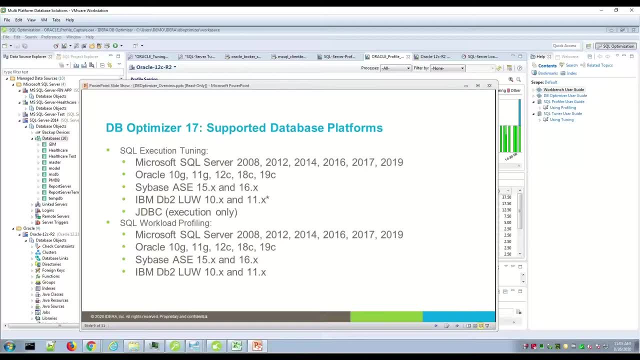 There's the four major platforms that I mentioned, and so you have some different ways of connecting there, And then you can see that the optimizers stay current with the latest versions of, say, Oracle and SQL Server, where you see Oracle 19 and SQL Server 2019.. 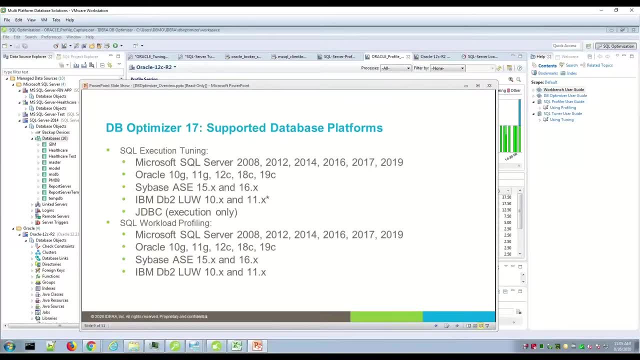 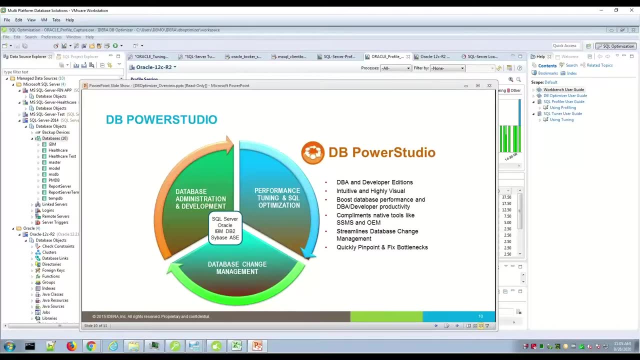 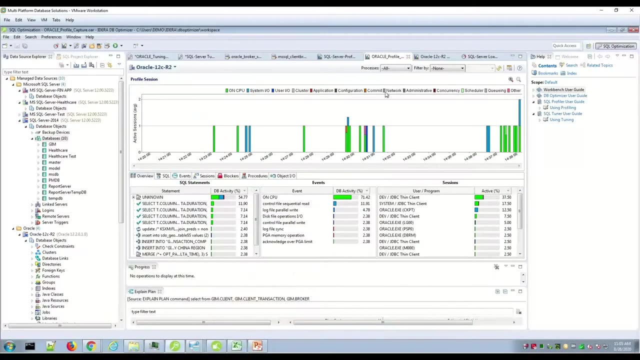 So those are the latest versions, and the new version of the PowerStudio bundles is on the way. So there's different ways of licensing the DB optimizer for you, And so let's dive into some of the examples that we have. Okay, And first maybe introduce the user interface. 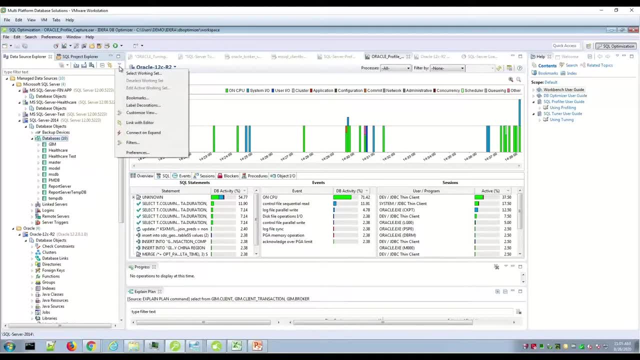 You have some flexibility here in terms of where you display these different menus, but on the left-hand side you can see my database explorer and then a SQL project explorer, And so these are just organization tools, where you'll start here with connecting and we'll dive into the connection window or registering the server. 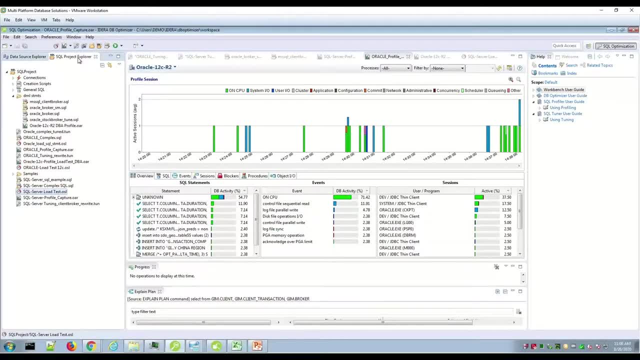 And then the SQL project explorer is a utility for grouping these DB optimizer files, and so here you can see some different examples of these, And if I just expand the dropdown you'll see these are different savable files in the DB optimizer, And so, again, we'll focus on the profiling and tuning. 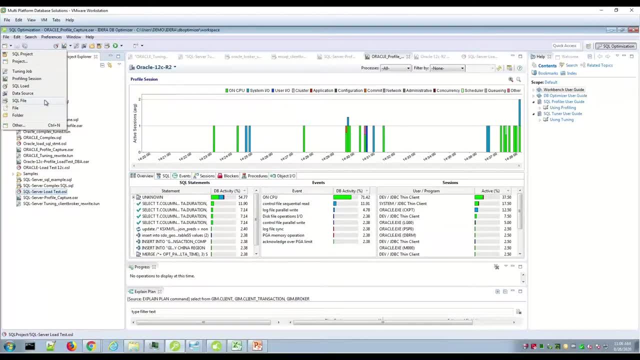 Those are the core areas of the tool, But if you want to start with a SQL statement and execute- that's where we'll start today- and look at the execution plan, And so the explain plan exists in the different database platforms, whether it's execution. 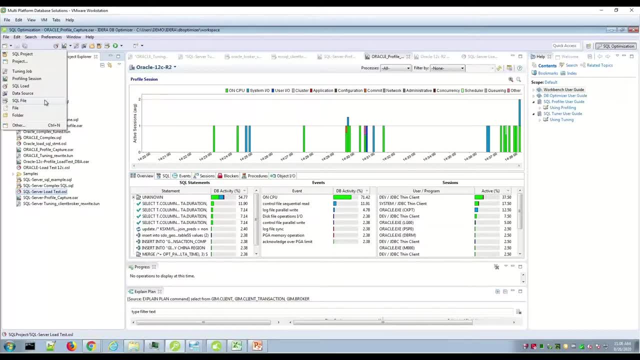 or execution plan or explain plan or show plan in Sybase right And then take that SQL into a tuning job. So we'll start with a SQL statement and bring it into a tuning window or, if you want to capture performance, we'll kick off a profiling session as well. 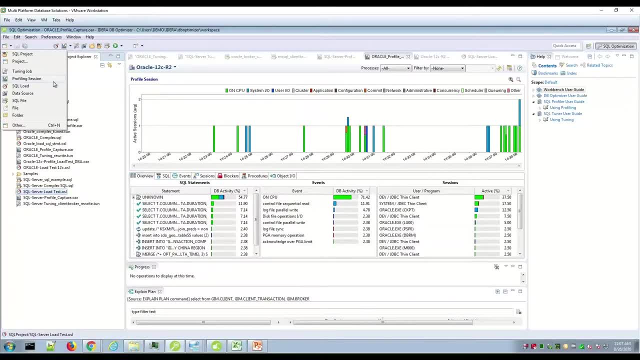 And so you have different starting points. Then there's some other utilities here. There's a SQL load utility, and so you can run transactions and execute multiple iterations of SQL to generate load and see how different variations of SQL perform with a higher volume or load test increase. 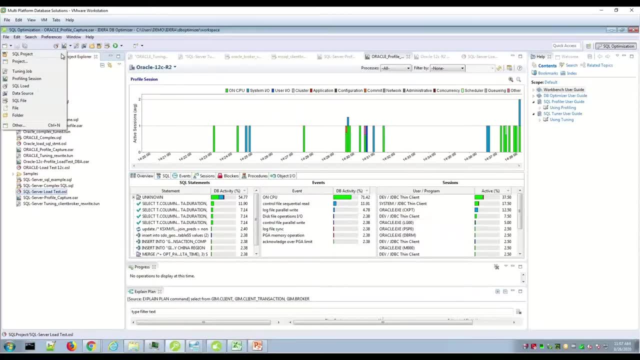 Okay, so you have icons here from the dropdown and then you can see those tied to the main toolbar as well, So you have some flexibility in terms of how to launch some of these windows or icons. Here's the dropdown window from the toolbar. 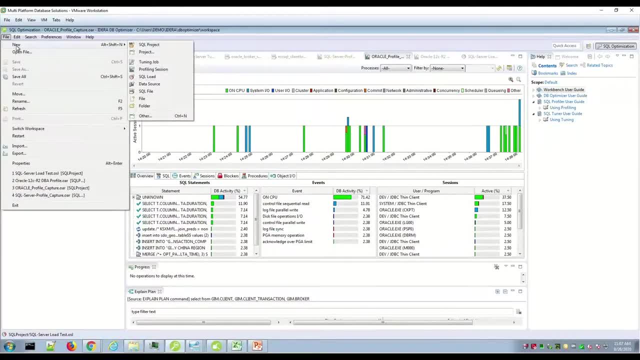 and then here's the file drill down, which has a similar file, new and those same options. So let's start with talking about connecting, and then the SQL Project Explorer is a way to organize these different files, and these are saveable, reusable files. 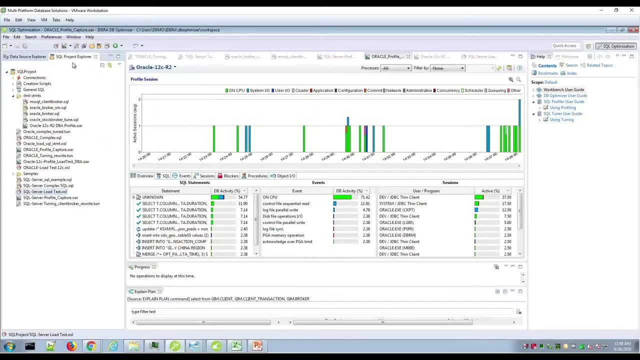 And then then you can organize those in different ways here in the SQL Project Explorer. So the starting point would be connecting to your different databases. You can see SQL Server and Oracle environments that I'm connected to here, And so you'll start here with the register. 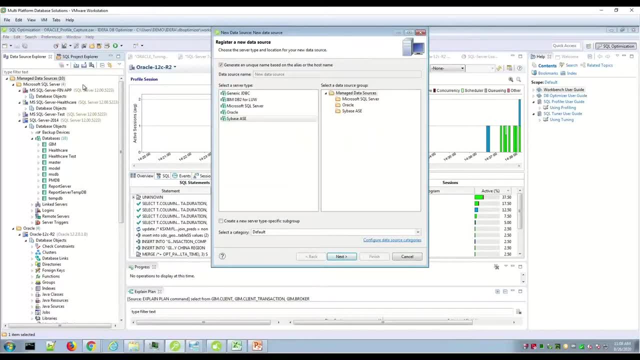 and this will show the user interface for connecting to your different databases. so you can see the big vendors there, where this tool started and now SQL Server and Oracle are probably the higher volume users of DB Optimizer in terms of the database platforms that this is used against. 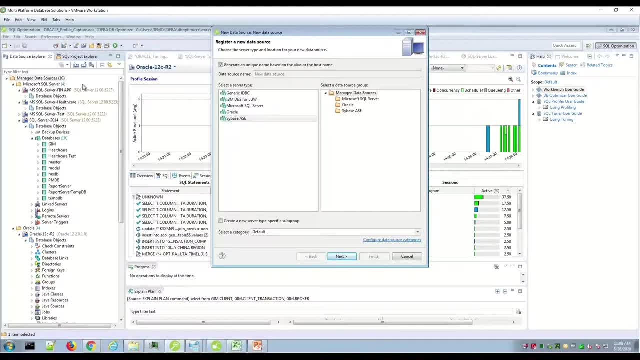 But Sybase, you know, still there, and some of the critical applications are remaining on Sybase, And so this is still widely used in the Sybase environment. And then, for today, the SQL Project Explorer is still there. If you want to use it again, you may want to start here. 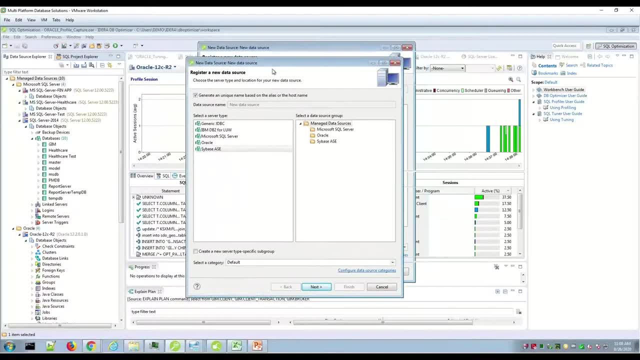 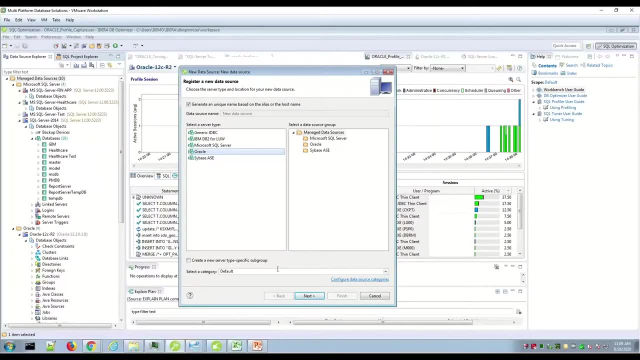 and then for today- you may want to start here- and then for next DB2, LUW, Linux, Linux Windows. that's the supported version. So this would be a wizard interface: choose your platform and then this would step you through. 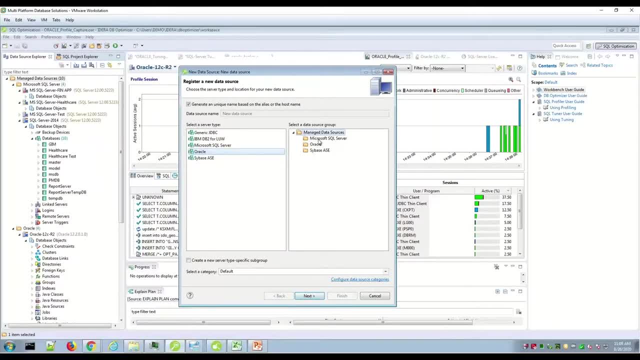 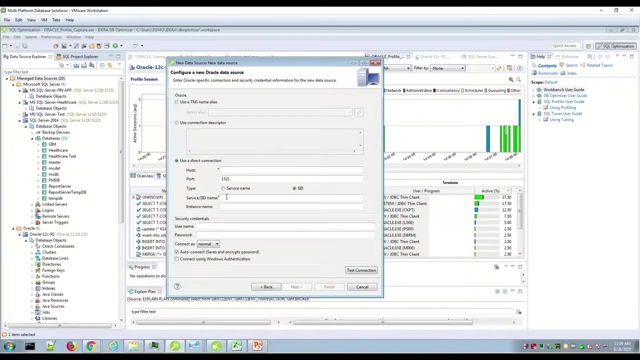 connecting and you have different ways of grouping or creating folders in different ways. So here I've just created a SQL Server folder, I created Oracle folder and I have my different connections grouped that way. So pretty straightforward wizard interface here. So here for Oracle, you can see asking for. 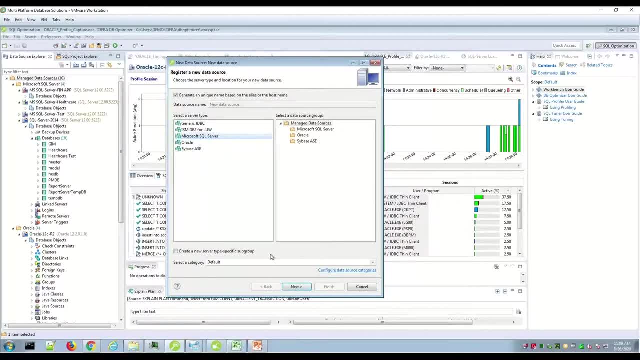 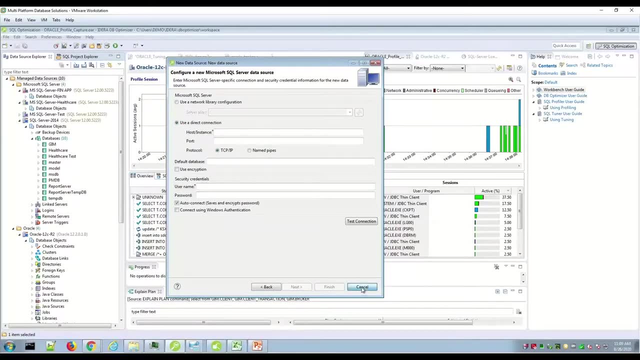 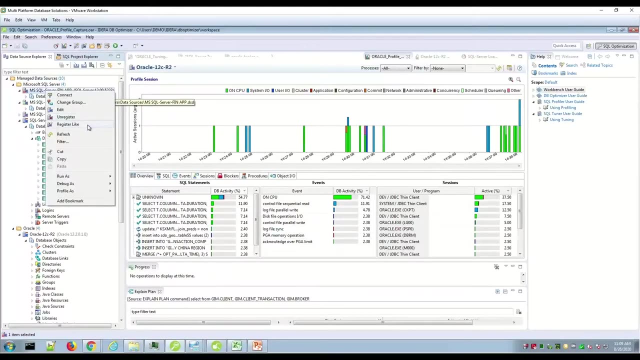 your SID or your instance Here. if I was to choose SQL Server, you can see it'll ask for your database and host, And so this is then saveable, and then you have different ways of even cloning these right. So right-click register, like would. 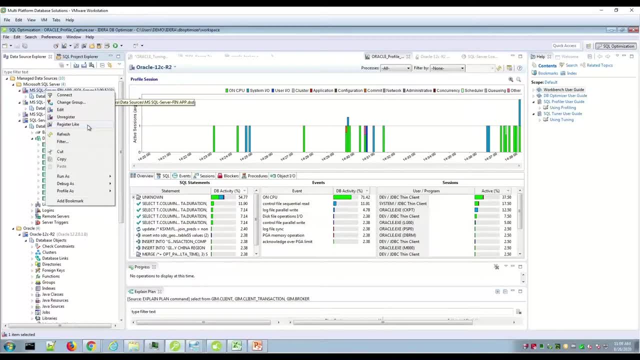 duplicate that connection and then you can perhaps change the database and so different ways of managing connections and duplicating those and naming those in a way that's convenient For you, so you can understand your navigation trait, Then you can explore right. so here here, if I maybe minimize the drill downs here, so for SQL Server, I 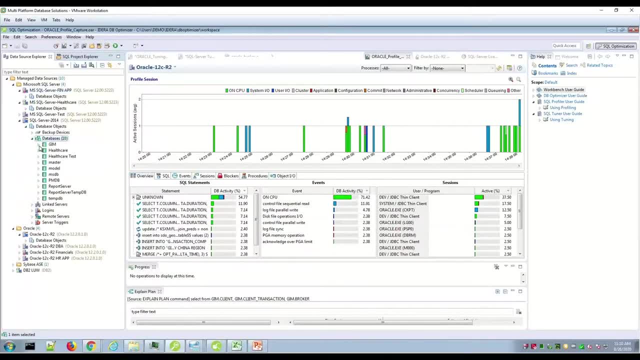 drill into database objects and then databases and so I can drill into my database tree and see my objects here and then more exploratory right. So here if I right-click, there's not not a lot of functionality here that falls, and maybe more the day-to-day products like 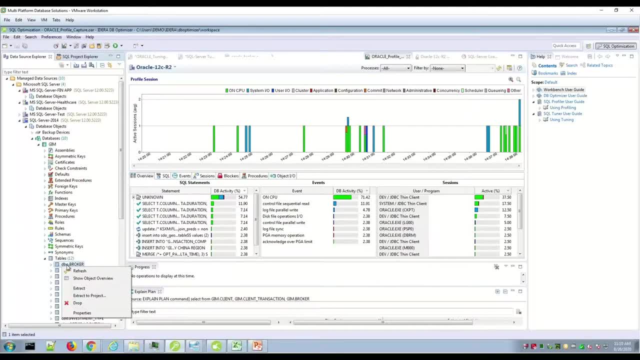 rapid sequel or DB artisan right. so the navigation tree is similar to those products but more just exploratory, so you can see which objects are out there and then use. you have that. you know, similarity with other platforms as well. so pretty extensive navigation tree for object support, but more exploratory here. 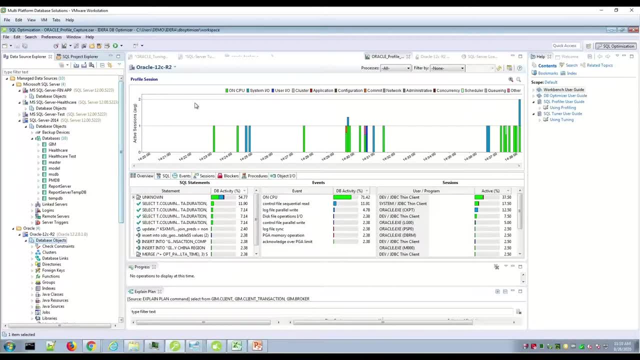 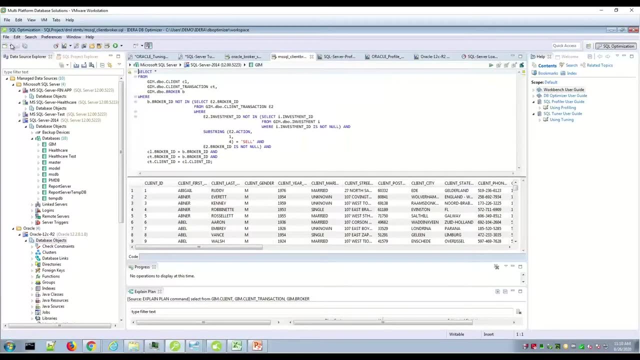 and then, depending on you know your starting point, you may dive into a different module or post a lot of different things you might want to take into account if you have a good connection, and then you don't want to have to have to do a lot of work on that and so on. just to show you how to do. 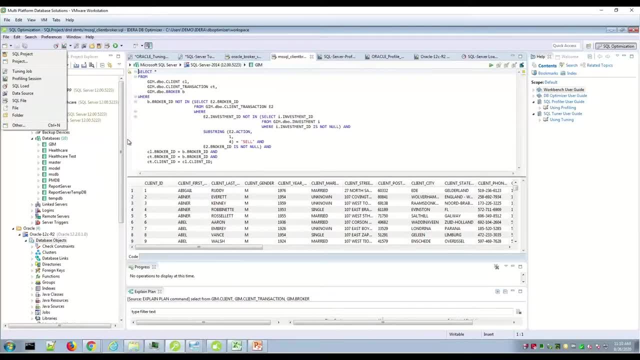 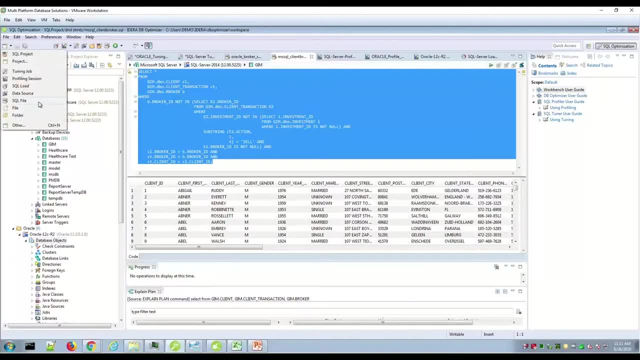 that. so I'm going to go to my dashboard and then I'll show you some of the stuff that I've shared in the previous videos, and then basically what I'll do, goal is to just go to my dashboard and go to a it's called the test data. 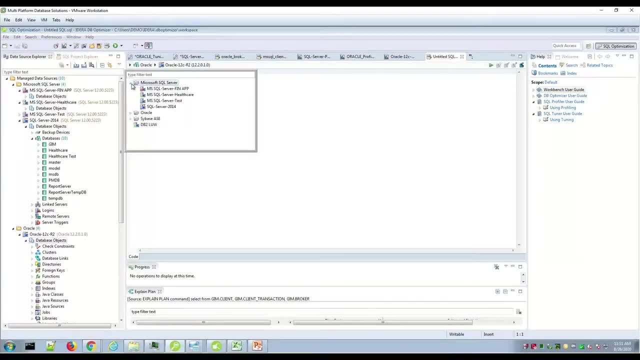 Uma, this is an overview of the web pages in the database and I'm going to go from here. just choose your database. you're going to see that I'm going to do, And then here I could just cut and paste a SQL statement and execute that. 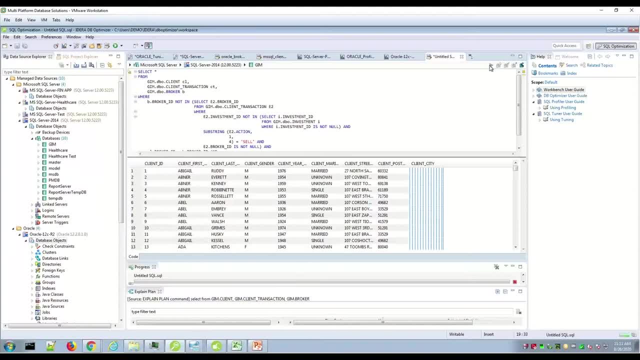 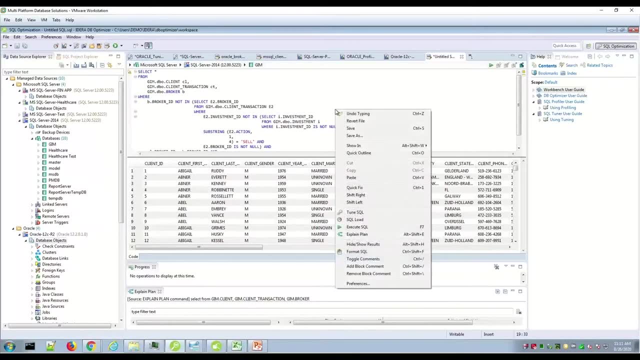 So you have the green run arrow in the top right, and so this would allow you to execute a statement, make sure you're connected properly to the database and then perhaps look at the execution plan, And so if I right-click after executing a statement, here's the explain plan. 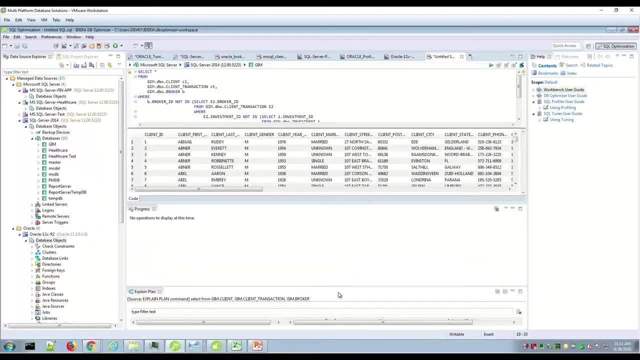 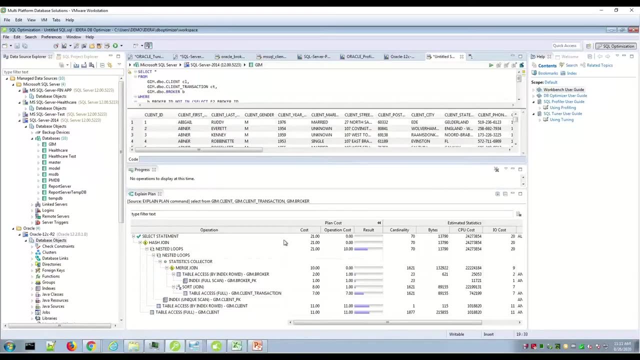 And so the lower portion of the screen would show your execution plan, and then you could double-click on that and expand that view. And so, for those of you that are newer to tuning, the execution plan exists in all databases in terms of seeing the path a database will take to execute that statement. 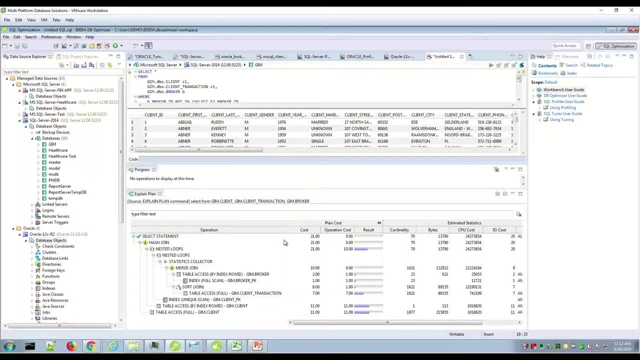 And so when you're looking at the cost of statements and the expense of statements, this is important to DBAs and people that are responsible for performance tuning. So here I could expand this. If I just double-click this window, you could see compatibility. 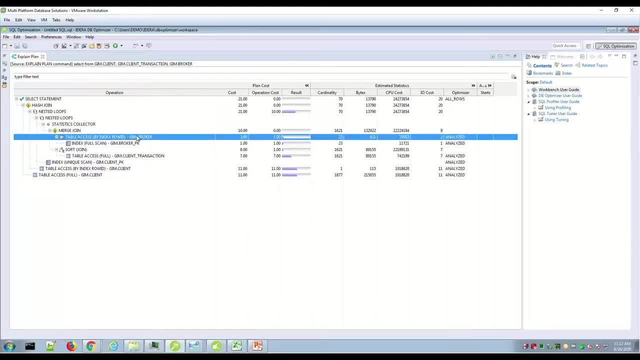 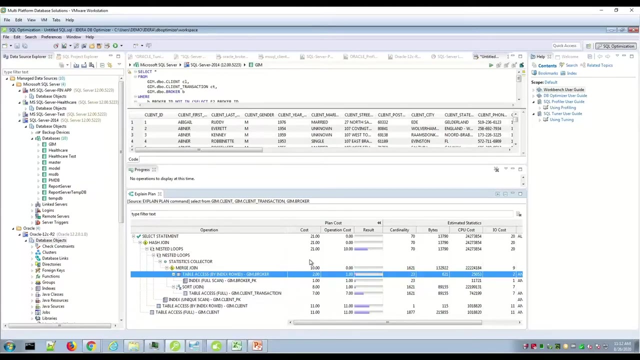 If I just double-click this window, you could see compatibility. So you have the graphical navigation tree of the different steps for the execution plan, And so you have that for different databases. Here's a SQL Server example And then a way to look at this, maybe in current terms or a simple comparison, would be similar to, say, Google Maps, right? 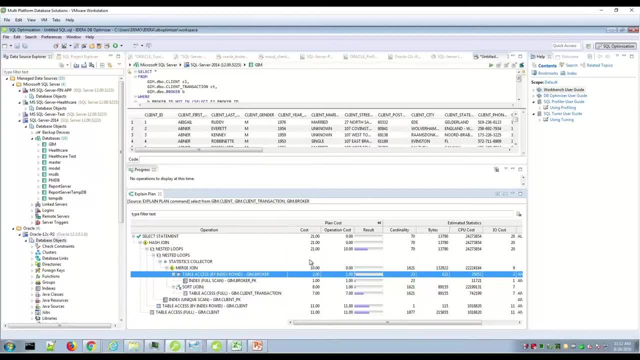 where you can explore different paths that you can take to get from point A to B, And so that's similar to the execution plan Where the database will show you the path it will take, based on rules in the database and statistics, right, And so, depending on, say, how many rows are in a database, it might influence how the database executes that statement, right. 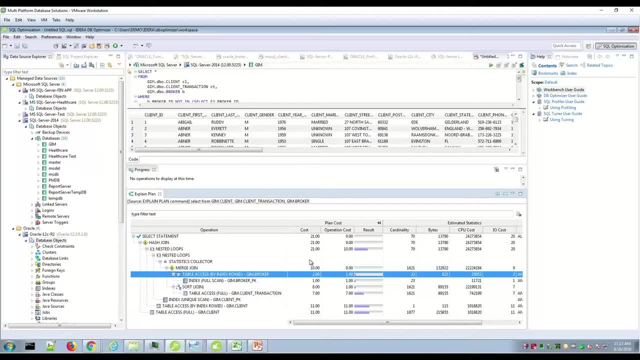 So if there's 10,000 rows versus a million rows, the database might take advantage of an execution path in a different way, And so that's what tuning and optimization is all about: right, Rewriting the statement And in a way that will improve the execution plan, right. 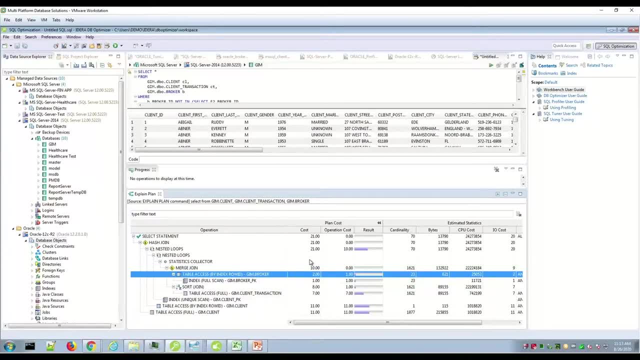 Because you could rewrite a statement and it doesn't improve the execution plan, And so that's the balance of tuning. So if you're familiar with execution plans, this should be helpful for you. But again, you have some different drill-down windows here. 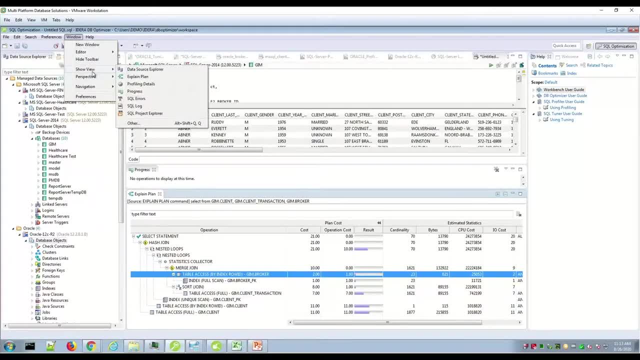 And so, depending on you- know your perspective, you can invoke or hide this explain plan window. And so under the window drill-down show view: these are different areas. If you lose a window or something hides that you didn't know how it hid, this is a way to bring it back. 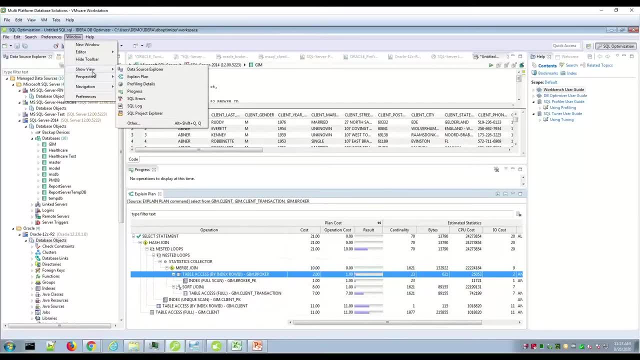 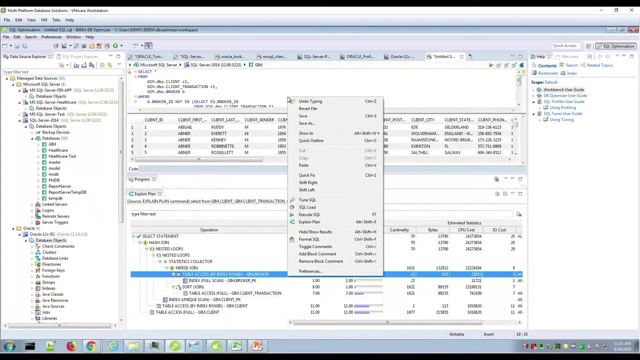 So just pointing that out. So the window explain plan: we'll bring that window back if you happen to close it. Okay, So from here we could take this statement into a tuning window, And so there's different ways to do that. 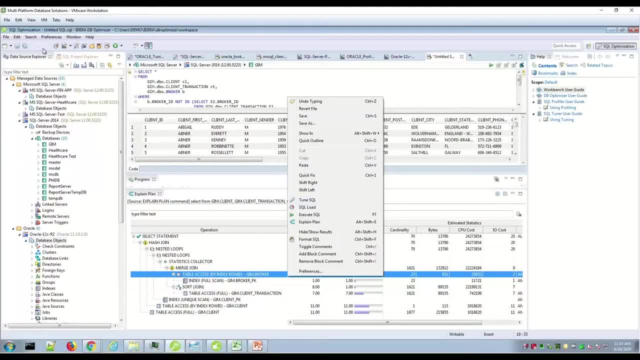 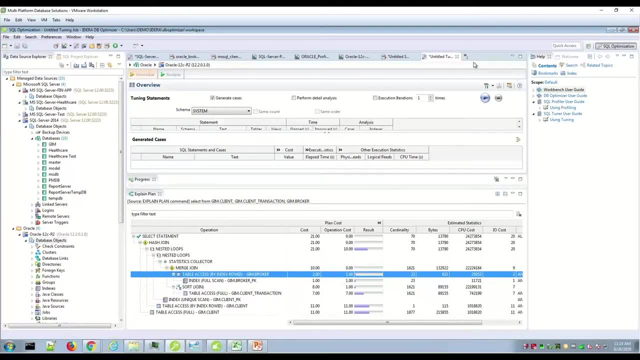 I could right-click and then there's the tune SQL, Or you could. You could invoke a new tuning window from the file menu. So file menu tuning job would open up a new tab And then this is the look and feel of the SQL tuning window. 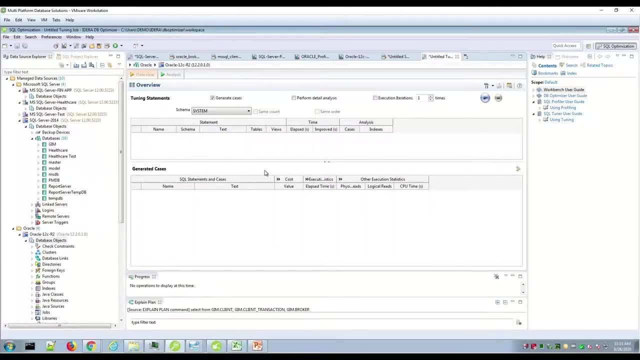 So here's a new SQL tuning window where you could just cut and paste a SQL statement here And then, as we invoke these different checkboxes, it would tune or optimize your SQL and generate rewrites and then execute those and perform iterations. So you can start with the tuning window. 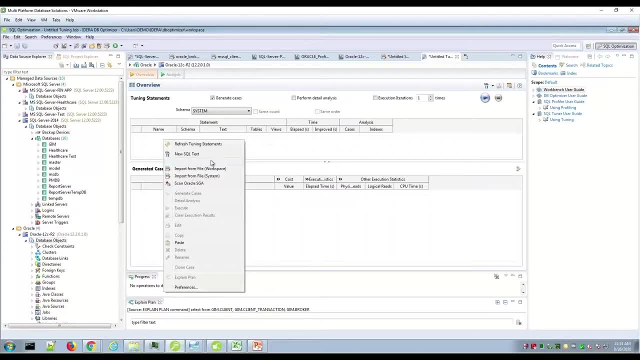 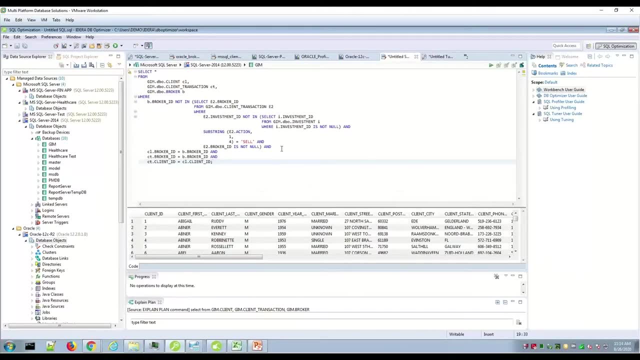 And bring a SQL statement just by right-clicking and you'll see different options there. Or if I go back to the SQL statement that we executed and we're looking at the execution plan, I can right-click here and then there's the tune SQL. 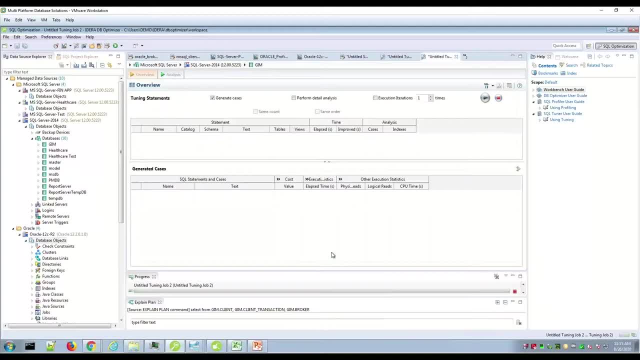 So just flexibility in terms of bringing statements from one window into another. You'll see that integration, And so now this opened up a tuning window with the SQL statement listed on the first row here and the top portion of the tuning window. So that's the tuning statements overview. 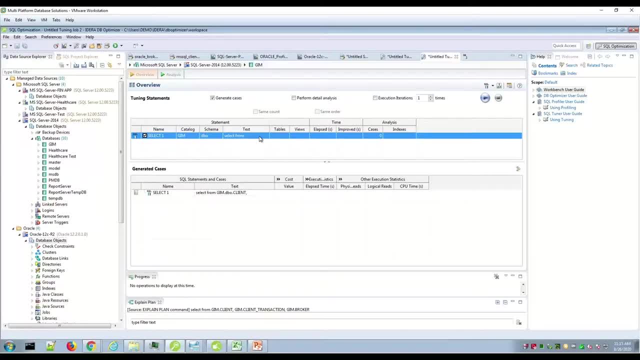 And then there's some different areas here that I'll point out before actually generating SQL rewrites, And then we'll be able to drill into the analysis tab and these columns will populate, And so that's where you have some flexibility in terms of what you'd like to generate. 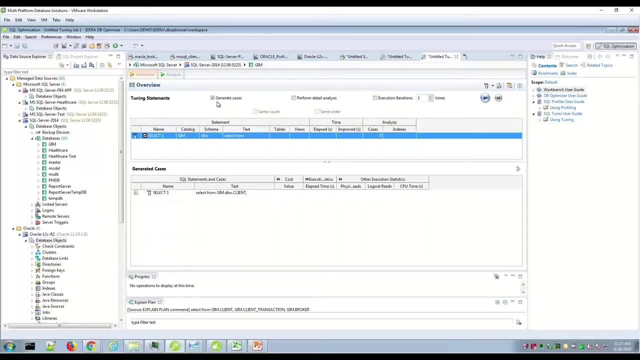 So you can generate alternatives in terms of SQL rewrites, Then you can perform a detailed analysis and compare those and find out what you'd like to generate, And then you can increase the number of iterations to, say, address caching right, So the more iterations would be a way to smooth out any variations in terms of the initial runs of caching. 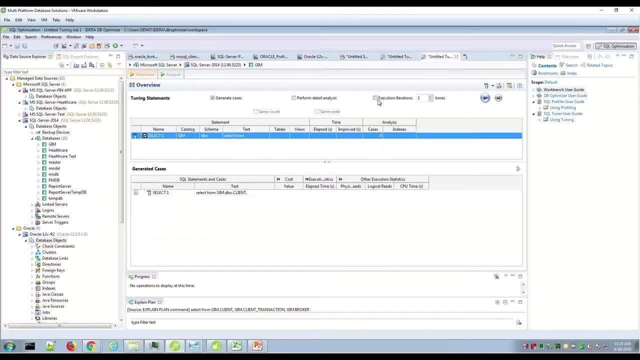 So usually it's recommended to increase iterations a couple of times, And then you have flexibility there in terms of comparisons of increase iterations And seeing perhaps where load testing can help. So we'll look at that as an example as well. Okay, so we just started by opening up a tuning or SQL statement window. 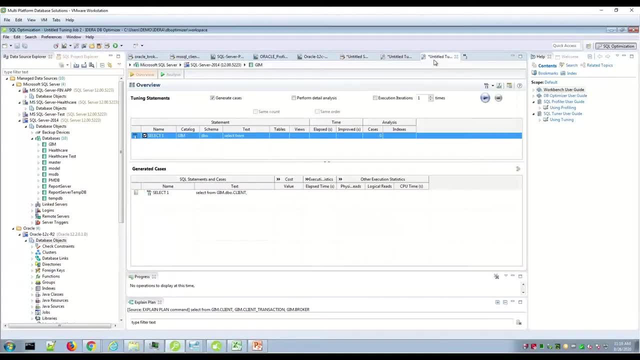 And then we brought that into a tuning window And now you have some options here where I can check to perform detailed analysis Here. I'll maybe increase the iterations a number of times And then here's the play button to set up the analysis. 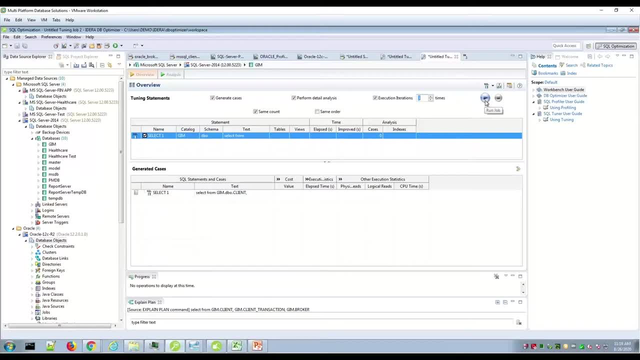 And then I can send this statement into the tuning window through the tuning algorithm. So here you have that similar green run arrow to execute a statement And then here's the play button to bring this statement through a tuning job. So if I kick this off now, the optimizer for SQL Server will build rewrites. 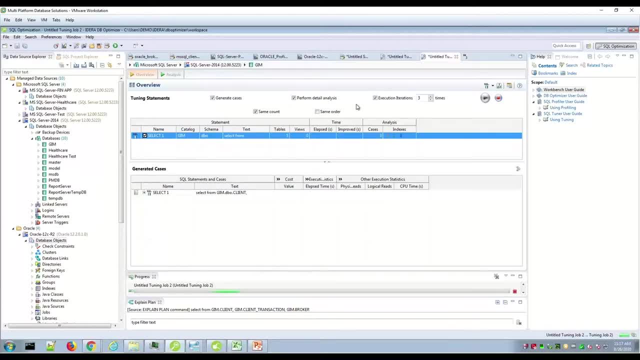 And then, in terms of the checkboxes that I have selected here, the detail analysis will actually execute these and then populate performance comparisons, And then you can visit the analysis tab to generate visual diagrams, do comparisons and then even generate a report or a summary report on the iterations. 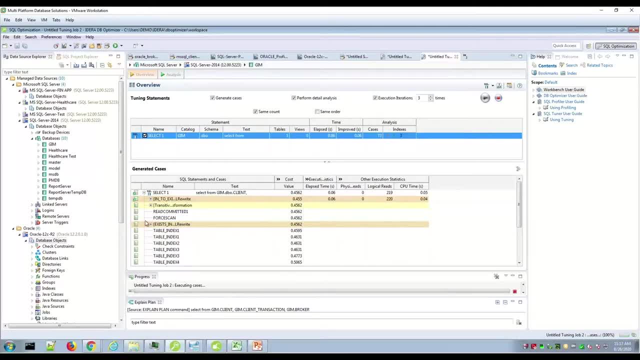 So there's a progress window. So that's chugging away there in the lower portion of my screen And you can see that as well here. Show view. So once you're familiar with the user interface, you can hide the progress window. 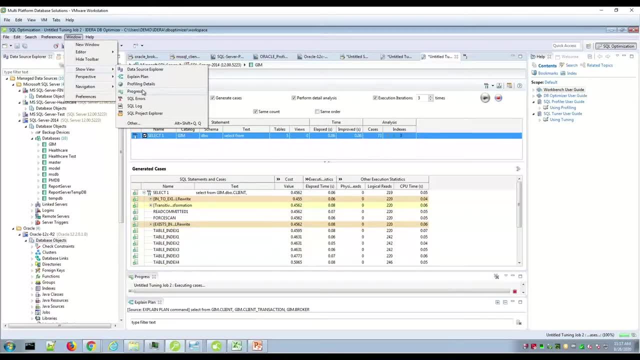 But sometimes it's helpful just to see what's being executed, And so now you can see, as I've let this run, first it generated the rewrites And then it started executing the alternatives, And now I have comparisons here and some summary information of what was generated. 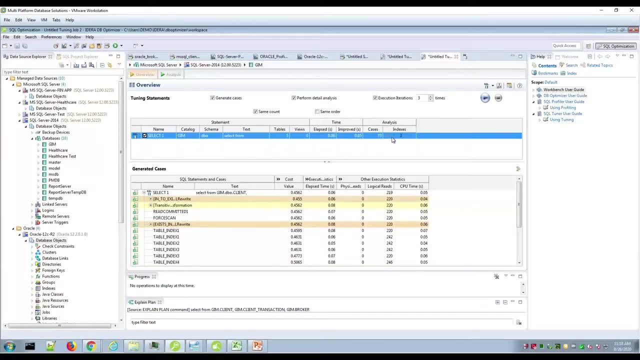 And so you can see it generated 73 different cases, And then there's an index analysis on the analysis, And then there's a different analysis tab as well. So here's some summary information- what objects were used, levels of improvement, And then you can drill down into these individually. 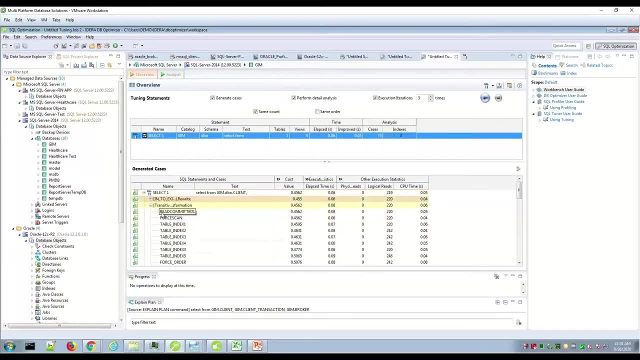 where can expand these alternatives and explore these And then if, depending on your level of tuning, you can mouse over and you'll see some summary information there, You can right-click and do comparisons to see how that rewrite compares to the original statement, and so you can see at the top there you have that original statement, same as the. 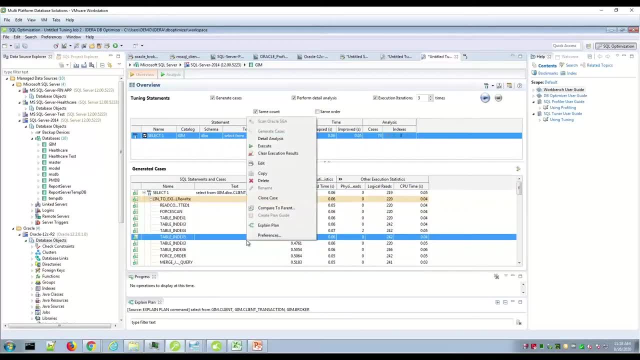 first line here and then here are the different alternatives. so if i right click on any of these, you can see where the optimization engine for that platform brought in, say a sql, sql optimization or a query hint. so here right click, compare to parent and you can do the side-by-side code analysis to. 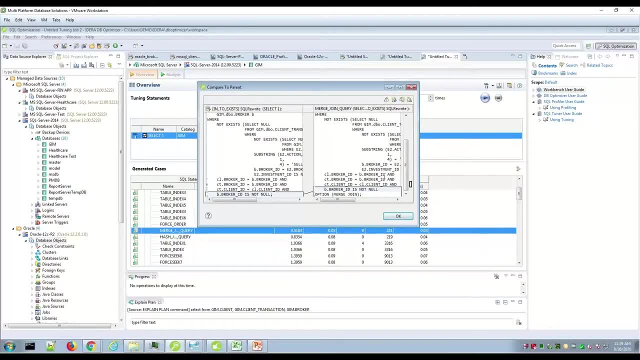 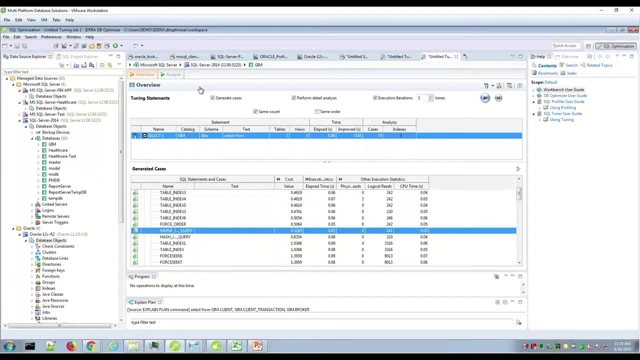 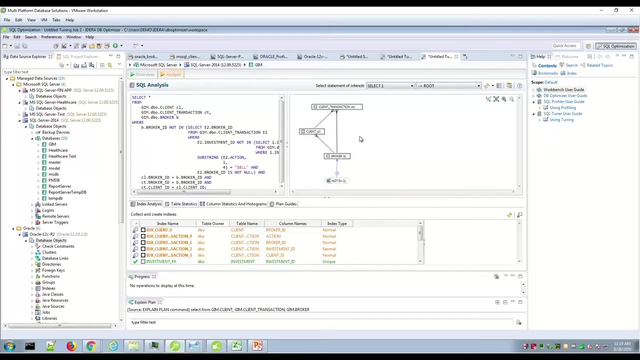 see where that sql rewrite occurred and and how it performs, so. so you have that side-by-side comparison in terms of code comparison, and then here on the analysis tab you have visual diagrams and then index recommendations, and so here you can see, at the top you have a drop down in terms of 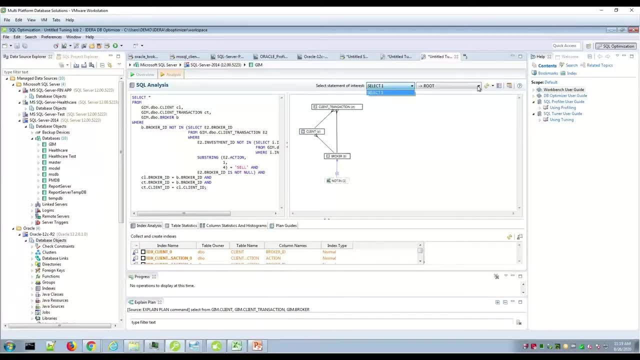 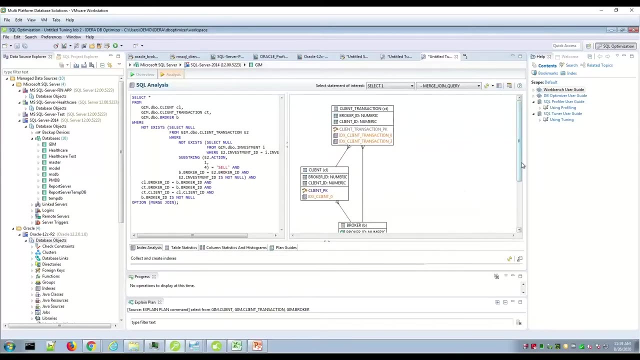 which statement you're looking at, right, so you can choose from the list of rewrites, and so that's. that's a similar list here. so maybe go back to that merge query- join. you can see the visual representation. right click- i have a detailed mode to expand the view here and then this is is a visual representation of this query. 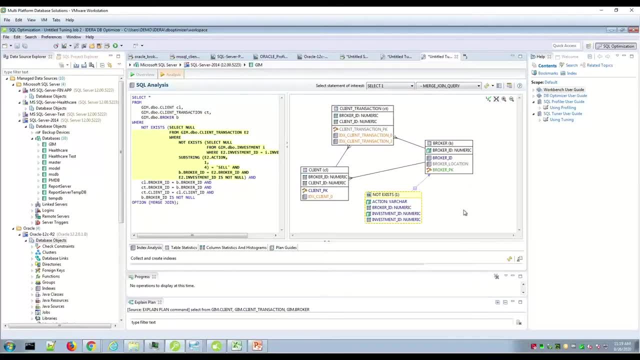 so not the execution plan diagram, but here i can actually highlight objects, indexes, tables, column level, and it will. it will point that out within the sql statement where that's being used, and so that's a benefit in terms of understanding sql and how the database is executing that. 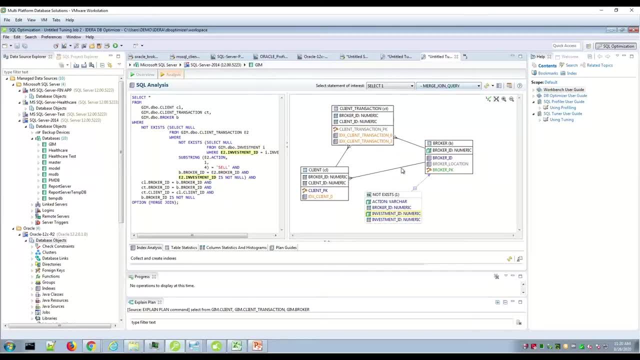 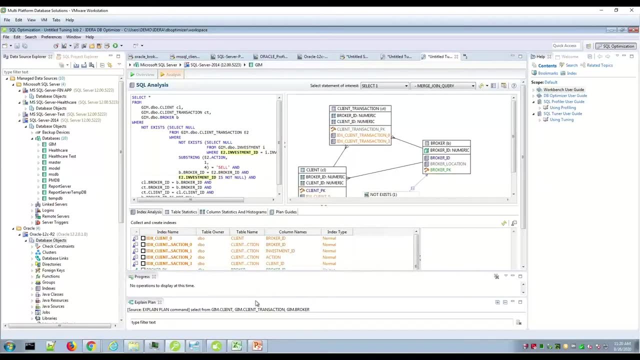 statement. and so you have that for any of these different alternatives, and then for the um, for the index analysis, you can see some different color coding and, and you can highlight those, let me hide some of these windows on the lower portion of the screen just to maximize. 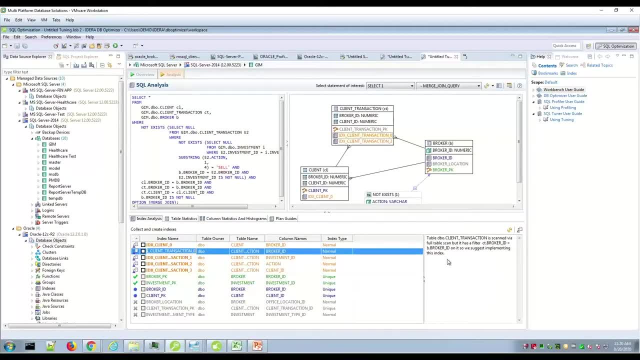 so, as you highlight one of these, you can see a summary of information here, and so black and the red is the index. as you can see this, when you are implementing indexing, i am going to do that that way. there are a few showing up here. like i said, betterRecordedClient. 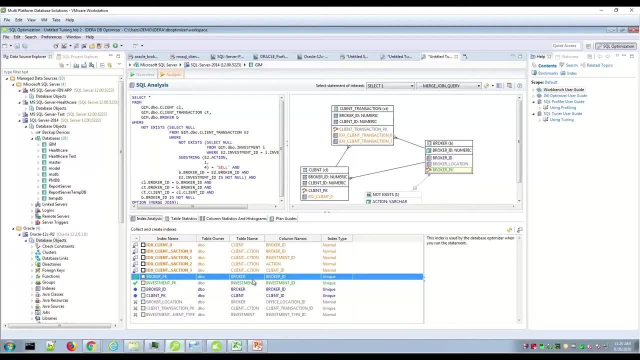 and text: 아이�ujuare~~ and the other key to the alguns. it should have been: if this are going to sufficiently Schmidt index and write the number for both the indexes and the others are going to be indexed and you can revise that so they are retained as you're implementing them, which is really important because it's going to change. you'll notice that you can reverse that if you want toеличre attends here or if you're usingходит, that's gonna be. you gonna see that right here. chan dm and your Page size boxes. Lets try this sorting index, redeem, indexed indexes. you can get one by that in the bottom. 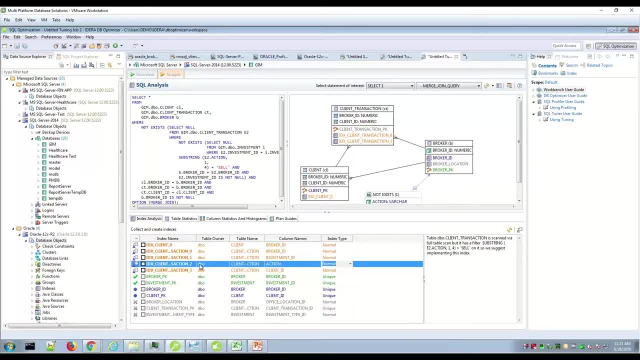 list of index indexes could mean one index for one index index. right and the green index index are actually being used by the sql statement or have an indexing strategy. you have the ability to generate the DDL for these alternatives. So, depending on your level of experience, you know there's performance with indexing. 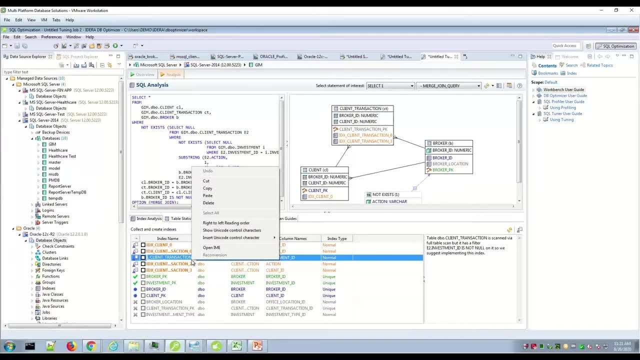 And so there's some considerations to have there. But you do have the ability to generate the DDL from this analysis tab. So in terms of implementing the SQL rewrites here, you can just double-click on these and then bring that into your source code. 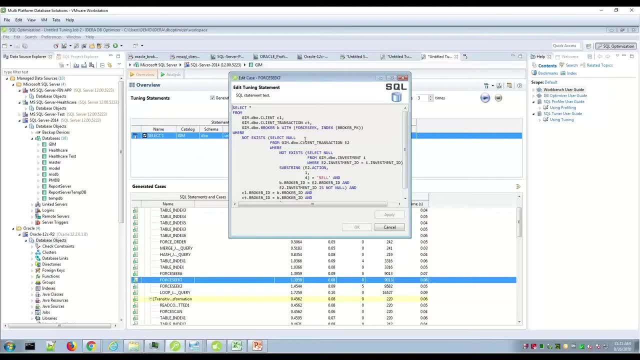 And so that would be a way to update or optimize the existing SQL. Again, if you're in vendor applications, you might have more of an indexing strategy if you're locked out of rewriting the SQL, And so that's where the profiling can be a starting point. 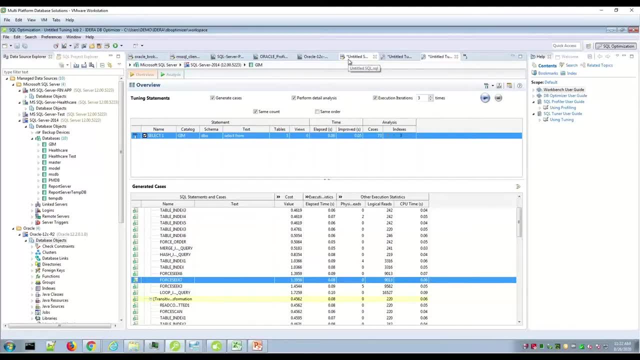 And so what we did here was start with the SQL statement and then bring that into a tuning session. So if you know what SQL you'd like to improve or optimize, you have that as a starting point. But maybe you're not as sure of what SQL is causing the performance hit. 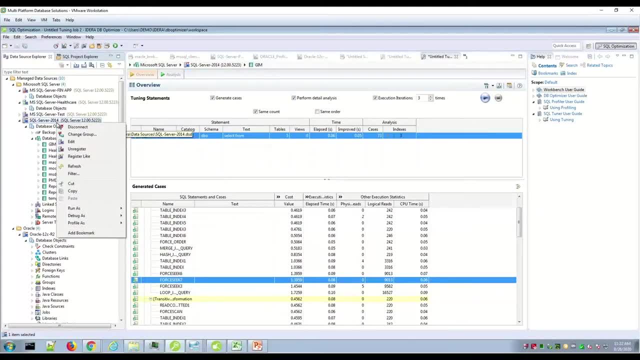 or you perhaps are just doing regular maintenance, And so that's where the profiling of your database is a benefit and a real strength of SQL Optimizer. So we'll close out with the profiling where this will do a collection Or capture of your SQL. 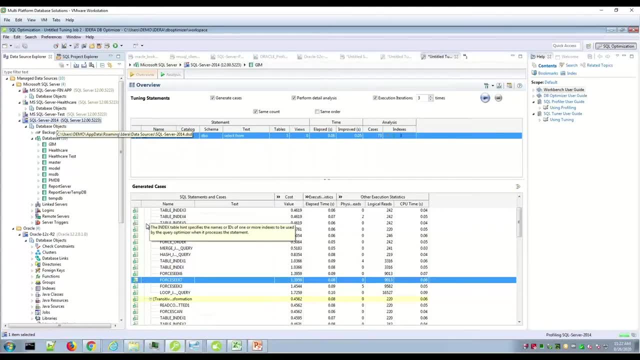 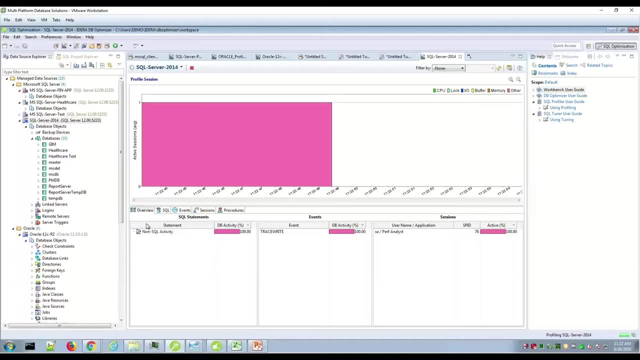 And so here I'll kick off a profiling session And you'll see now a collection of SQL transactions And so let me kick off a little activity here just to generate some spikes here. So we mentioned DB Optimizer is part of a standalone product. 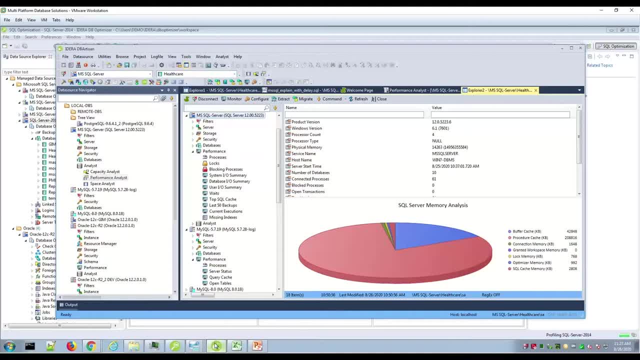 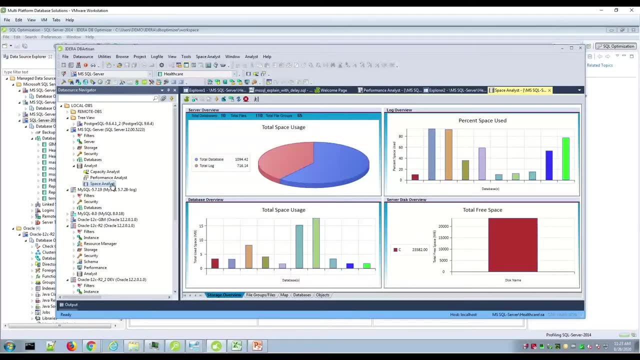 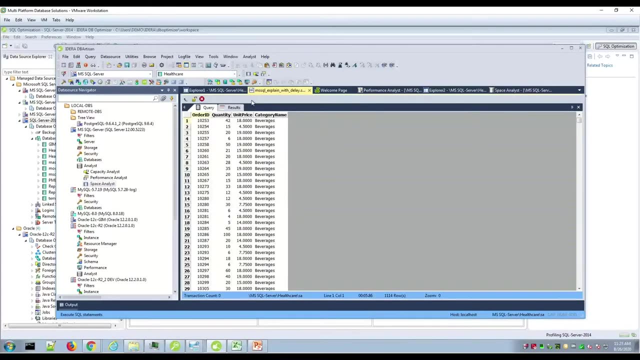 but also part of the Power Studio bundle, And so DB Artisan is a well-known tool there, And so here, if I maybe just generate some activity here within this database that I'm collecting, we'll generate some performance spikes. So I'm just in DB Artisan here executing some SQL. 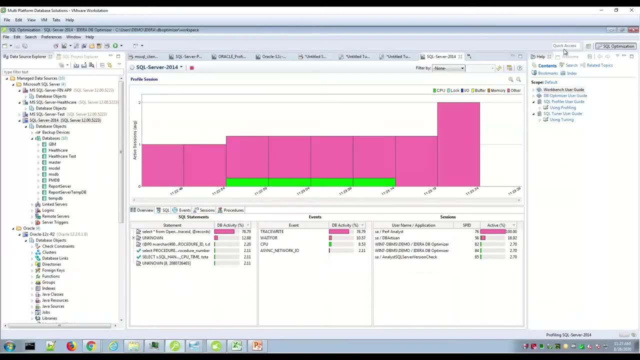 clicking on some performance metrics, And so that will generate a performance spike. So here you can see DB Artisan as an application that is starting to collect SQL from. And then another area within SQL Optimizer is the- let me kick off a load test here as well to generate activity. 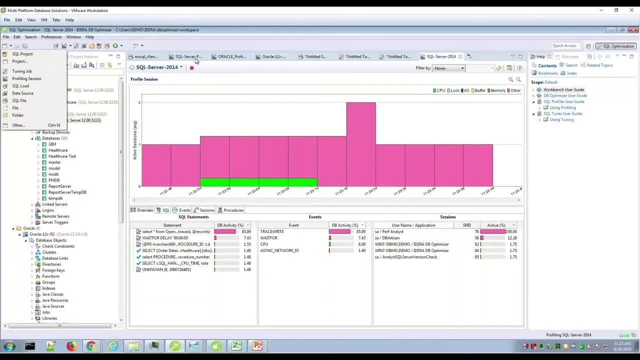 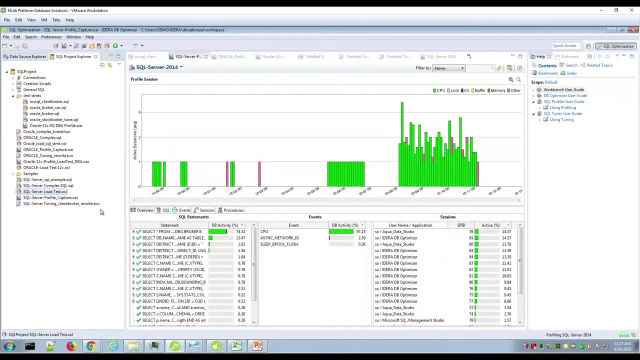 And so, again, these are different utilities that you can take advantage of within DB Optimizer. So there's different file extensions for these. right? So you can see: the profiling has the AR extension, the tuning has a tun extension, So the load testing has a. 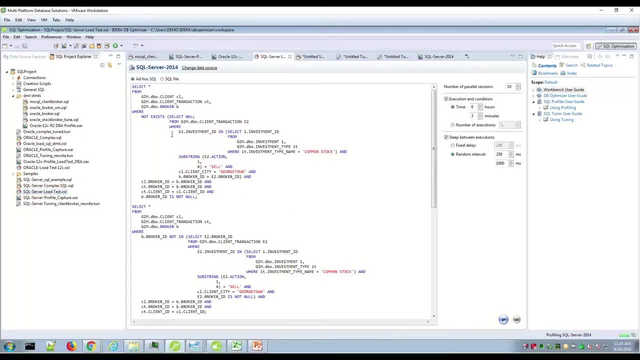 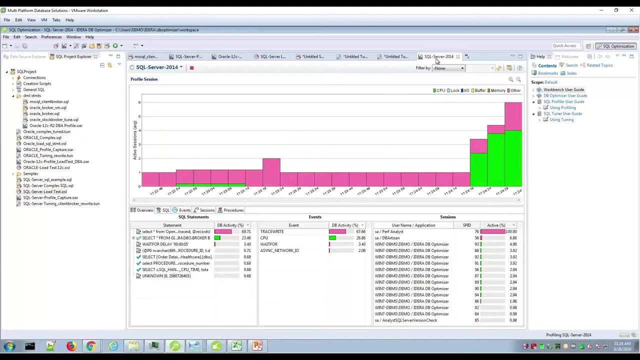 and so here I have the ability to execute one or multiple SQL and then increase the number of executions or parallel sessions, And so I'll do that here And then again go back to this profiling. So this is a capture right. You can see it's running and collecting. 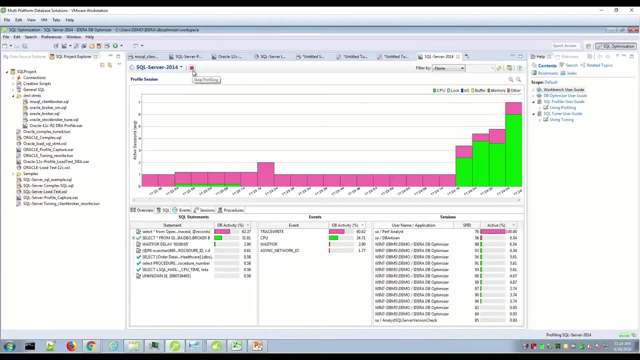 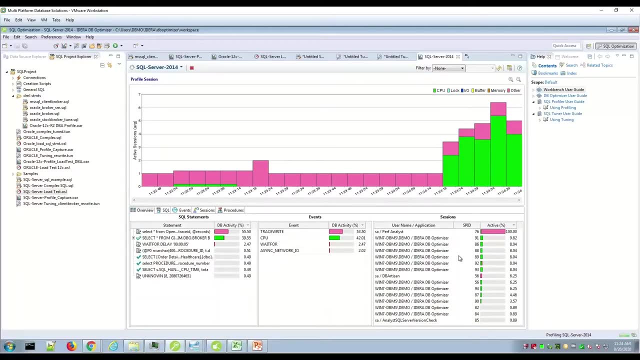 I have the stop icon there that would stop the collection, But we'll let this run a little longer So you can see some of the different transactions that it's collecting. And then you have a drill down capability here So you can see overview of the SQL statements and then the performance spikes. 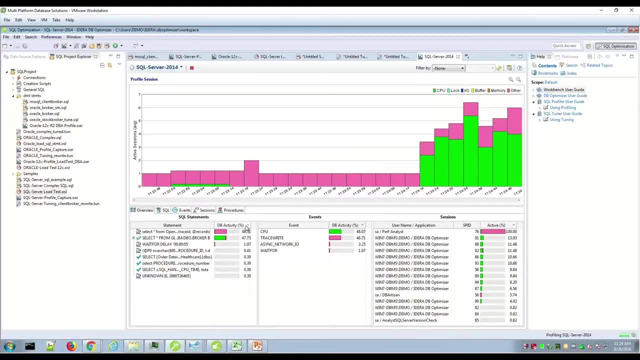 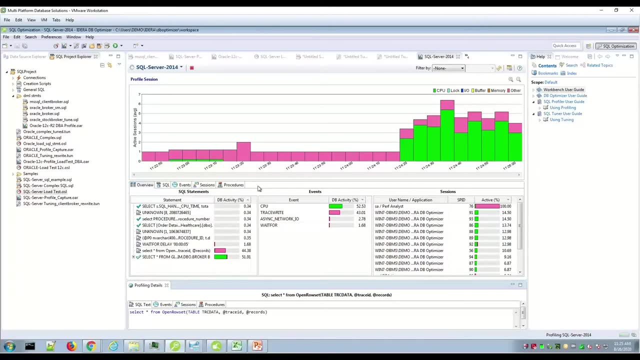 And so there's color coding here, breakdown that you can explore or isolate, And then you have these different tabs as well. So you have the SQL tab- events, sessions and procedures. So this is a great utility for for finding out what's going on in the database, right. 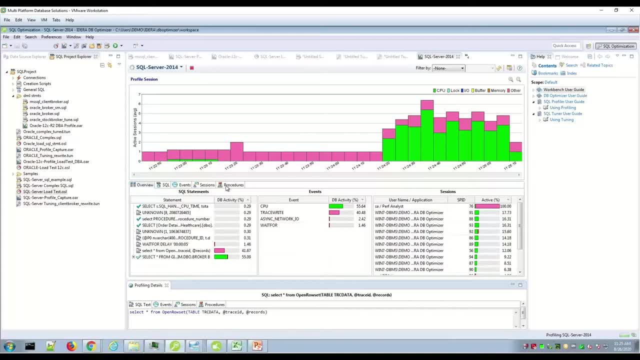 If the database is taking a performance hit, let's kick off a profiling session or, you know, in terms of regular maintenance, let's just see what's going on in the database, And so you wouldn't leave this running 24 seven. 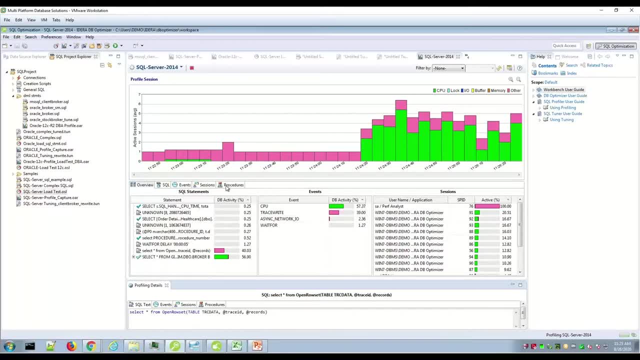 but it's, it's a way to capture and collect. So if you have a certain time of day that perhaps the database slows down, that would be an area that you can explore, Um, or you know, in terms of regular maintenance right. 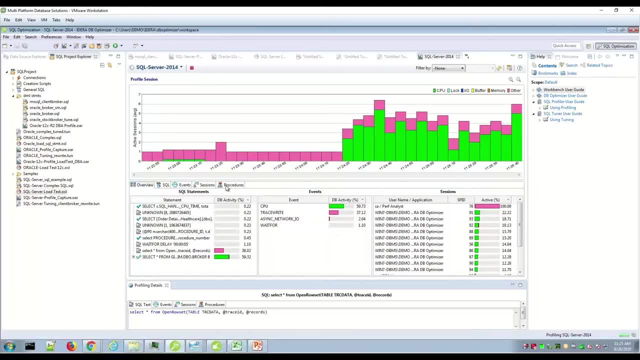 Like we all, we all have automobiles that we have to take care of, right, And so, of course, there's a problem. You, you, you lift up the hood and you have to look at the engine, uh, or in terms of regular checkup, right, 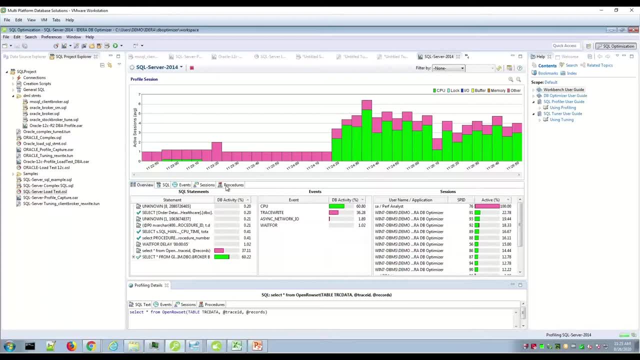 You, you, you. you lift the hood and see what's going on inside of the automobile, And so that's what you can do here with the profiling session, And then you'd stop this and save this. So you can, you can save this over time. compare this to other databases. 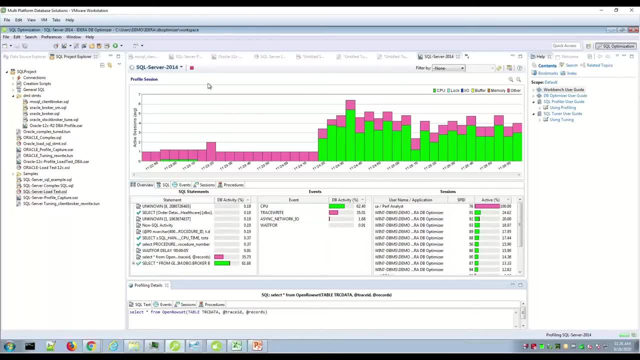 Um. and so Here's a sandbox environment where, uh, I'm performing this and say SQL server, Um, and then I'll. I'll stop this and we'll drill down into this. but here, if I switch to some of my other environments in the sandbox, here's: 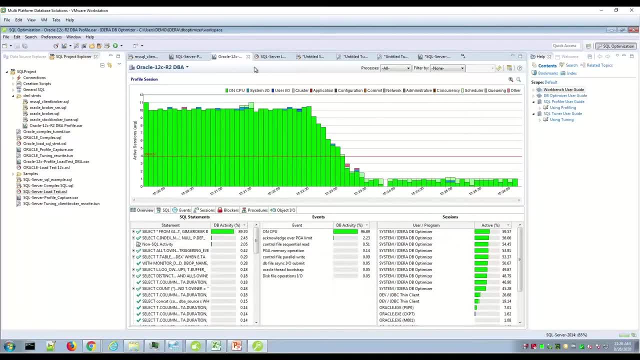 here's an Oracle collection, right, And so um very helpful, especially if you're managing multiple platforms. uh, to do this from a single tool, um is is powerful, right, And you'd have to spend time configuring this for different database platforms. 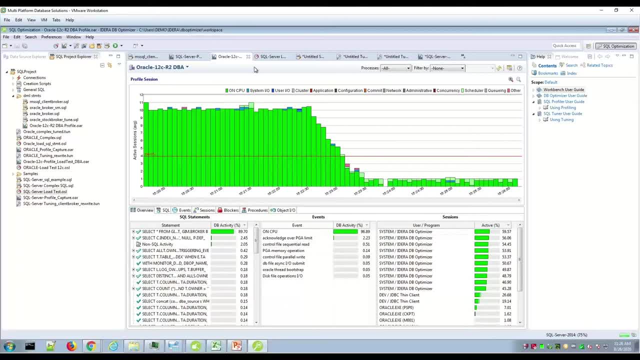 depending on the, the, the tool you're using. So, for the four major vendor platforms, uh, this has been proven technology. And um, depending on these different areas, uh, the, you know this. this is: this might be the critical area in that DB optimizer that you use. 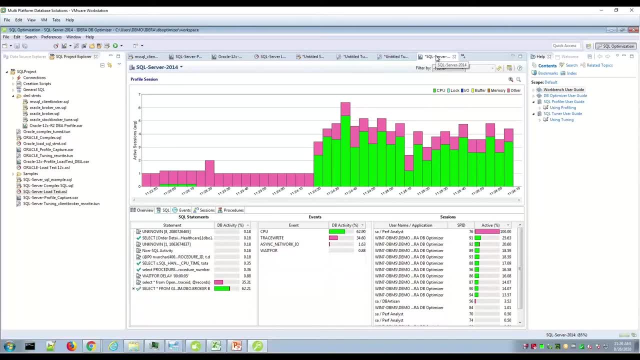 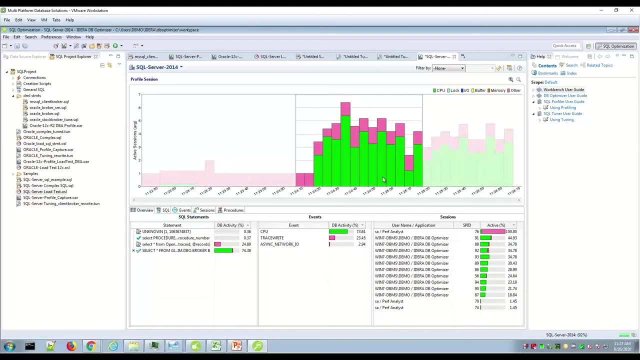 Maybe if you have junior um developers or folks newer to tuning they, they focus on the tuning SQL and testing SQL and learning SQL that way. So DBAs uh appreciate this profiling capability. Um, so here I could, I could mouse over a certain window of transactions and it will isolate those for me. 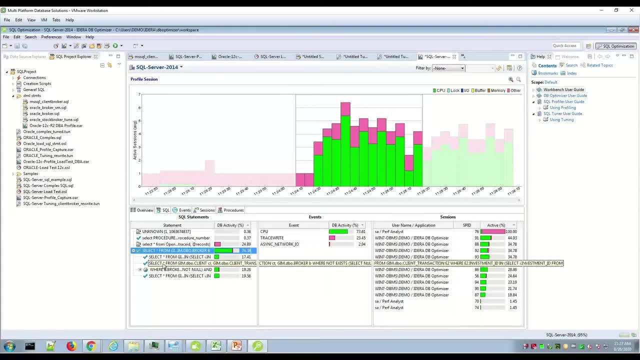 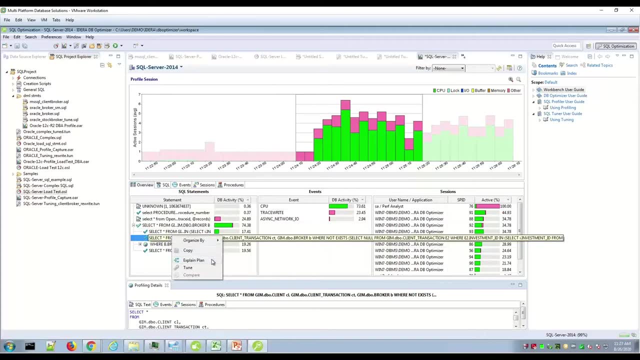 Then you can drill down into those individual transactions And then, if I right, click from here, this is where you'd see the integration to those two areas that we started with, the execution plan window or the tuning SQL right, And so you have different navigation points. uh, within DB optimizer. 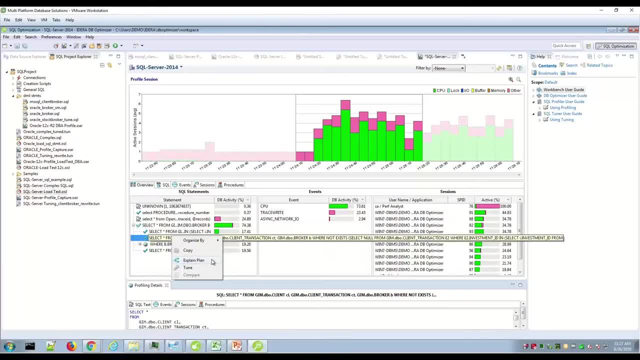 whether you're starting with a SQL statement and then bring that into the tuning window, or if you start here with the profiling, drill down into an individual SQL that was collected and then bring that into a tuning window. Um, so the the tabs here are helpful. 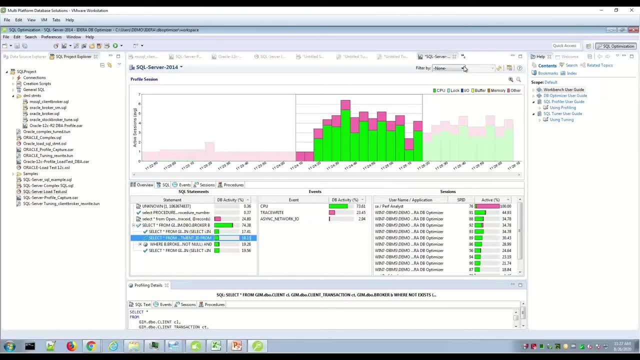 Here's a just overview with the performance spikes and then you can. you can start filtering here, Um, here, if I just unclick here, um, you have a filter where I could say, all right, just filter and show transactions just from certain applications or database. 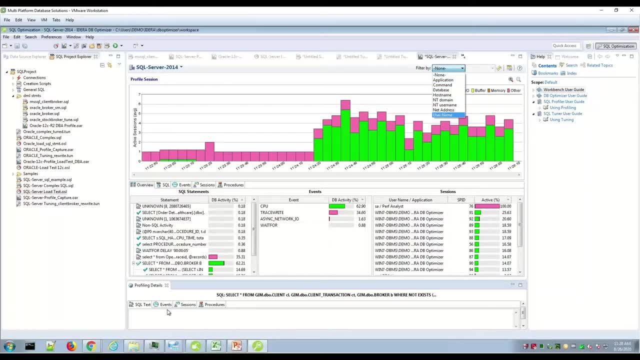 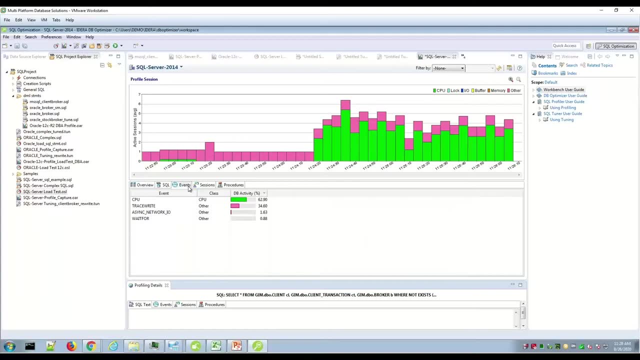 a certain user, right? So these are helpful drill down areas. Uh, and then you have events sessions and stored procedures, right? So events will group and show the color coding of the database activity and you can sort in different ways and see what that event wait was for. 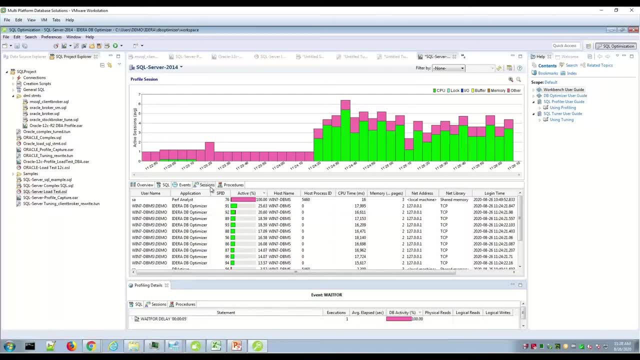 Okay. so again, we were trying to bring some momentum to these products, um, and we're building new versions of the power studio bundle, And so we want to thank everybody for joining Um. we had a few slides here in terms of: 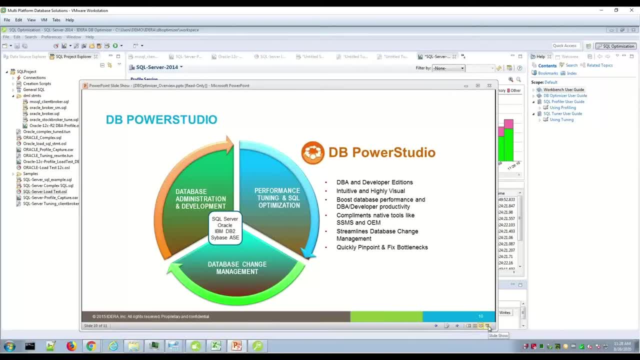 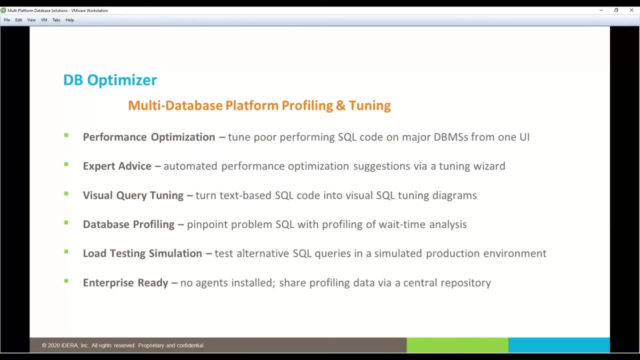 um, just where this product fits. um, that might be helpful to, to to understand, And so, um again, these are the areas that we focused on in terms of where the database optimizer helps. Um, these are the different platforms and supports. 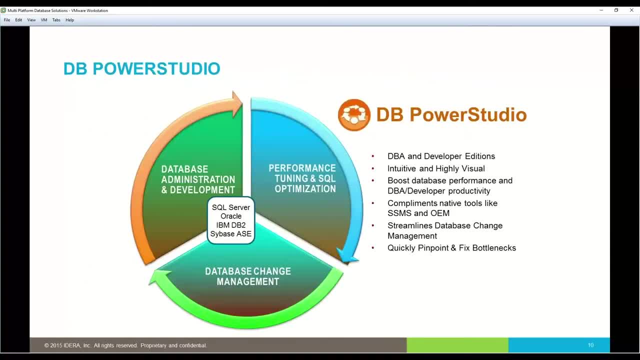 and then it can be licensed in different ways where it's uh, it's part of a uh individual product line or uh the bundle for developers or DBAs, And so, uh, the DBA edition would be to say DB artisan and power studio and the change manager product. 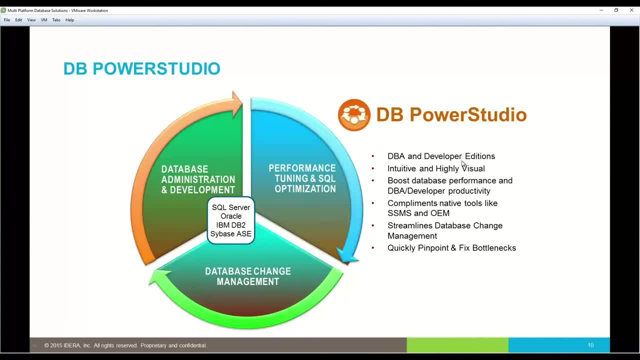 The developer edition would be rapid sequel and DB power studio and the change manager product. So look for future webcasts on those areas, right? So today was DB optimizer, tuning and database performance. Uh, we'll have upcoming webcasts on DB artisan and rapid sequel, and then change manager will probably be merged in those.